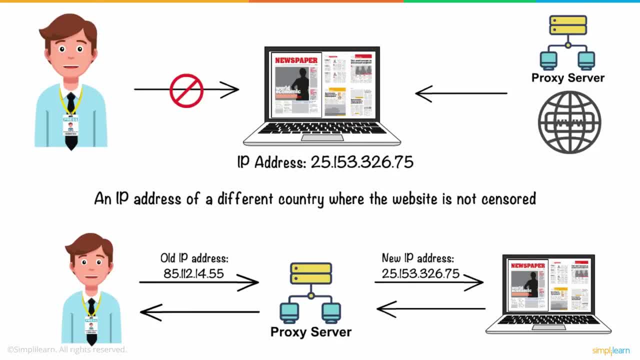 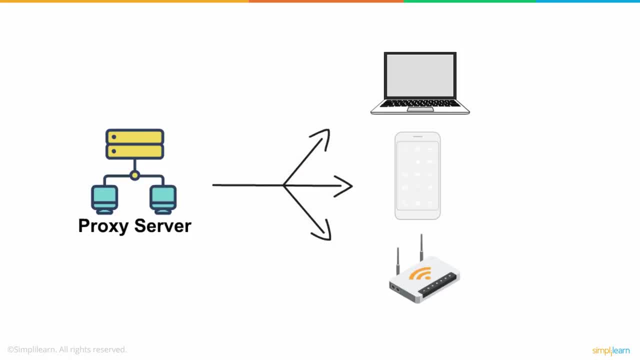 It's passed on to Jonathan's system via the same channel. Regarding accessibility to proxy servers, you must first set it up on your computer device or network. Next check the steps required for your computer or network, as each operating system has its 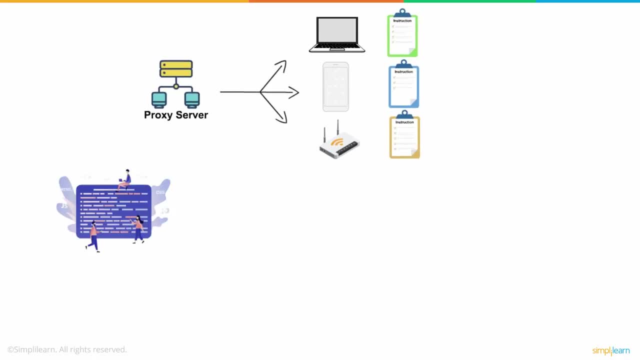 setup procedures. In most cases, however, setup entails using an automated configuration script. There are plenty of free proxy services available on the internet. However, the safety of such proxies is rarely verified. Most free proxies will provide an IP address and a relevant port for connection purposes. 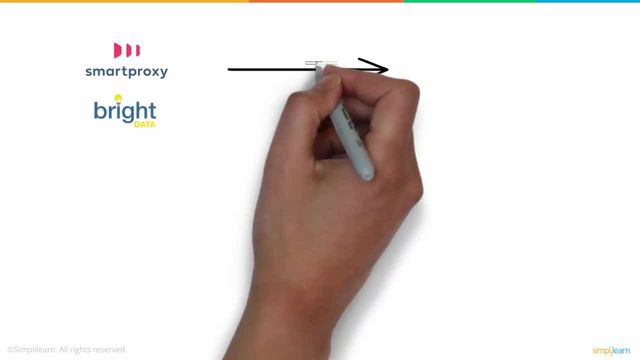 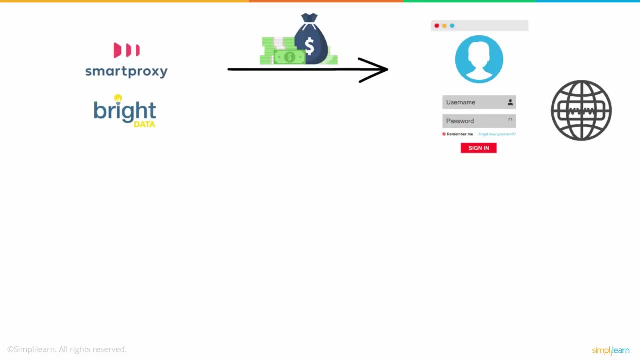 Reputed proxy providers like Smart Proxy and BrightData that run on subscription models will most likely provide credentials to log into when establishing the connection. This extra step acts as authentication that verifies an existing subscription on the proxy provider's server. unlike free providers that are open to all, 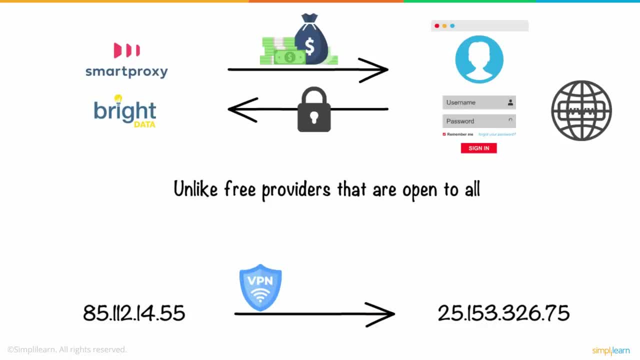 When it comes to hiding IP addresses, many people consider a VPN to be the primary solution. While that's true up to some extent, there are a few things proxies do differently. In the case of VPNs, extra encryption is also carried out to create a secure tunnel between. 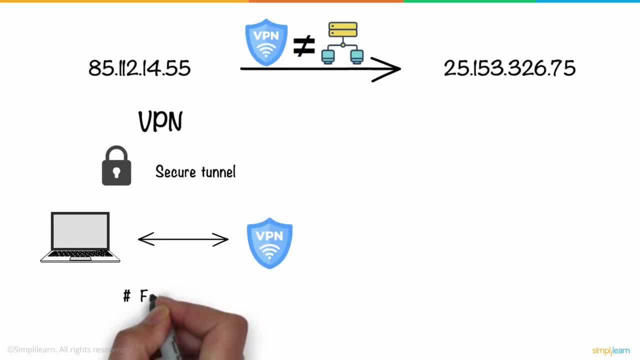 the user's device and a VPN server. A VPN is usually much faster, more secure thanks to multiple layers of encryption, and has little to no downtime. Proxies tend to be comparatively unsafe, With the service owners having the exact IP address of the end-user and having no. 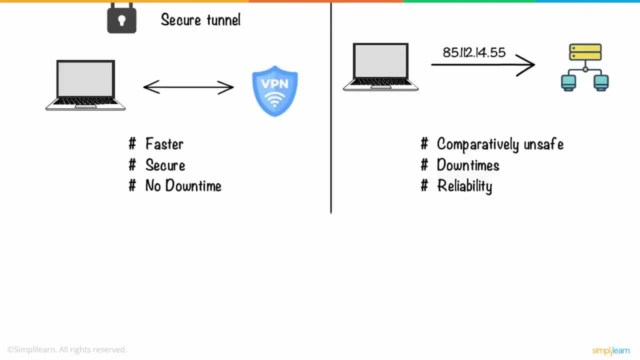 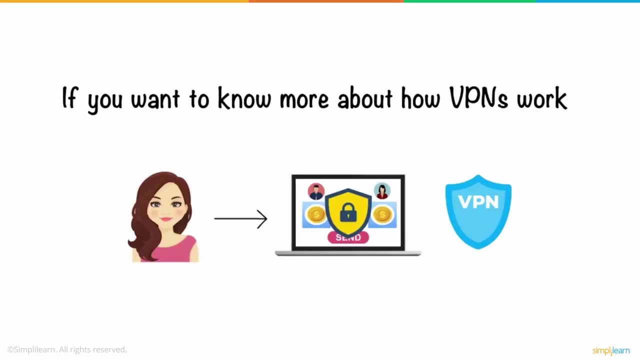 guarantees regarding downtimes and reliability. If you want to know more about how VPNs work, do watch how Jude could have protected her banking credentials using VPNs in our detailed video linked above. Now let's take a small quiz to check how much we have learned. 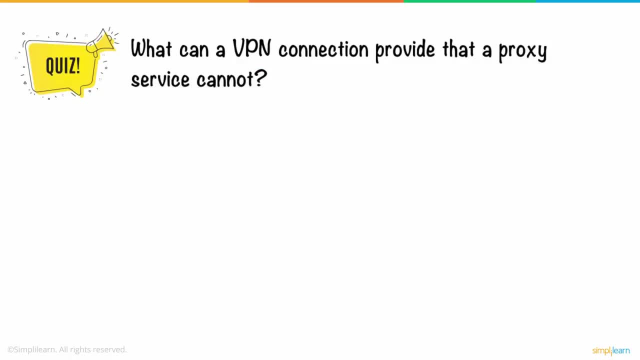 What can a VPN connection provide that a proxy service cannot? A New IP address. B- Multiple layers of encryption. C- Access to geo-blocked content. D- Authentication credentials. Think about it and leave your answers below in the comment section, and three lucky winners. 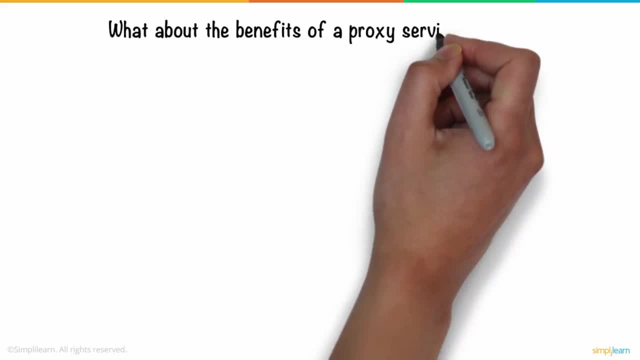 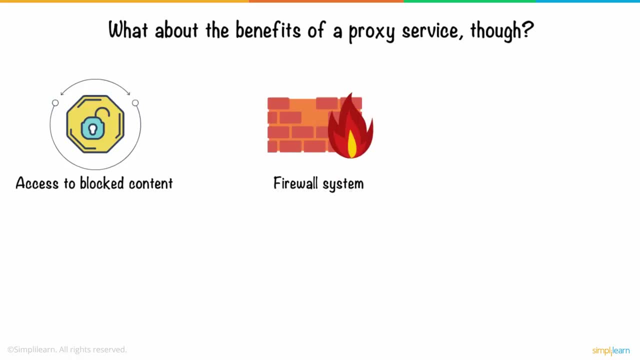 will receive Amazon gift vouchers. What about the benefits of a proxy service, though? Besides allowing access to blocked content, proxies can serve as an efficient firewall system. They can also filter content from third-party websites, allowing control over internet usage. In many cases, browsing specific websites can be an advantage.